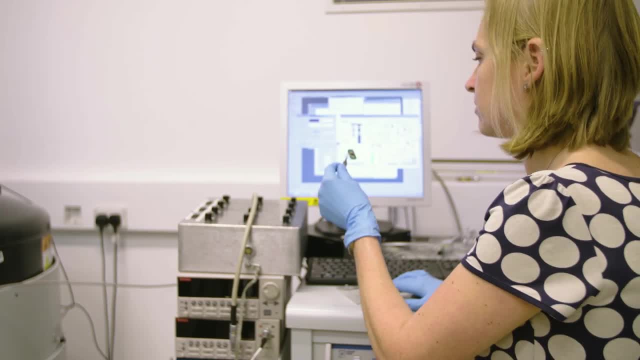 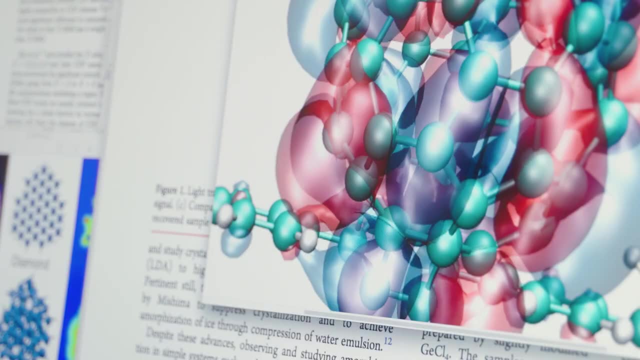 how we thought. The materials course at Imperial is delivered by 35 or so academics as well as a whole range of talented teachers. We have a number of teaching staff and we encompass the whole ensemble of materials. We draw them together in the first two years where we get this fundamental understanding. that's across the whole. 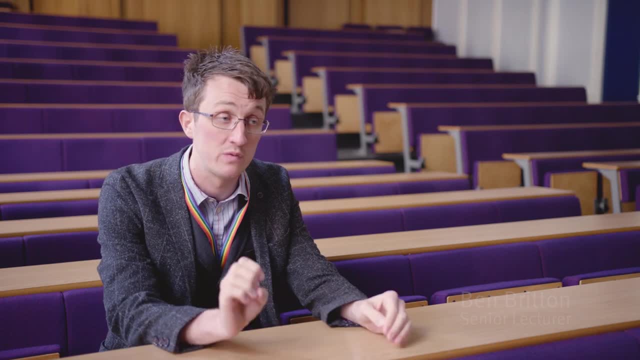 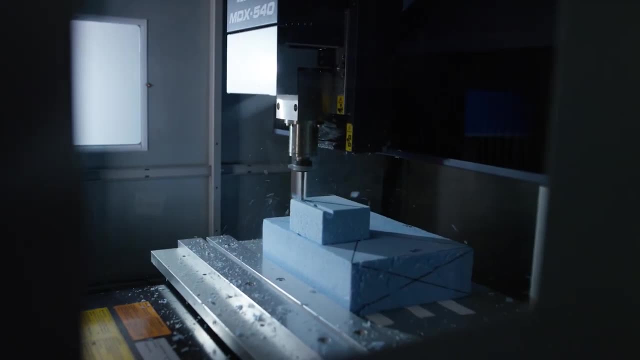 of our discipline And then in the last two years of the undergraduate course, we then specialize in specific core courses that you would elect to choose and using those to highlight and develop ideas and theories that will help you use these skills in the workplace. The facilities in the 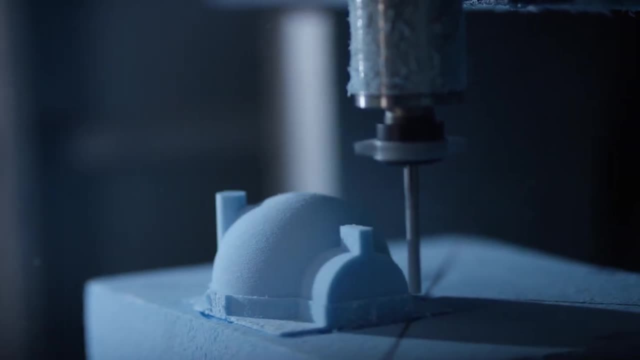 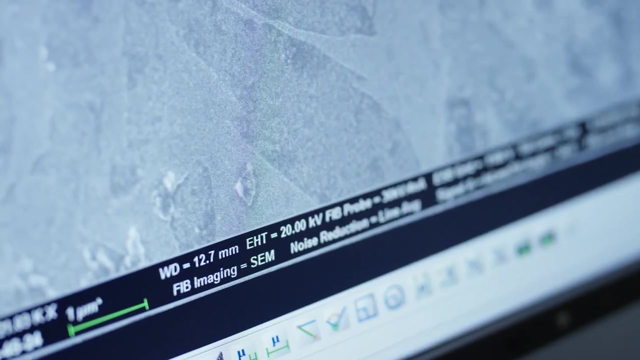 Department of Materials are cutting edge. We have a dedicated lab specifically for our fourth year research students that has x-ray instruments, It has electron microscopes, It has atomic force microscopy. Then we have cutting edge approaches to interpret that data And so combining 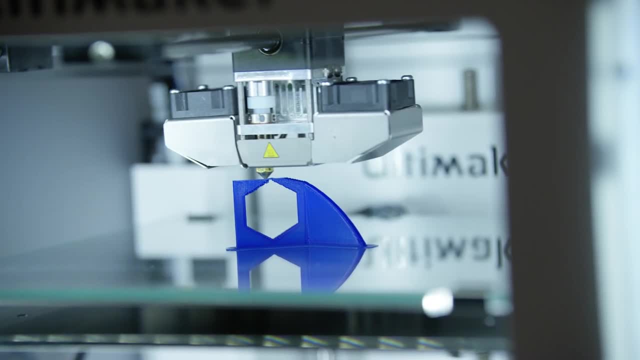 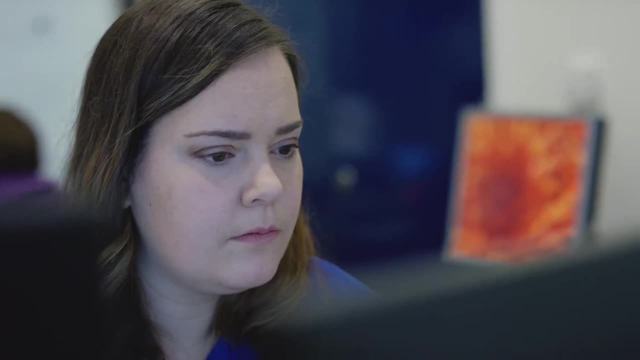 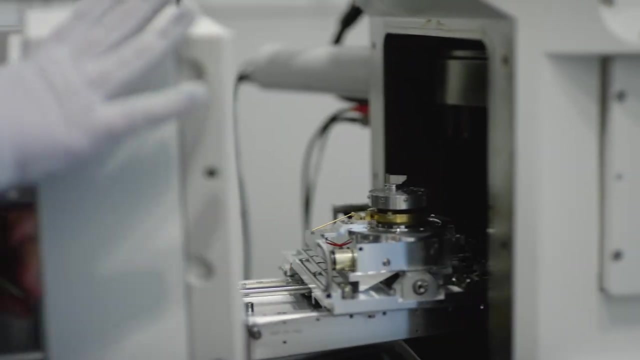 those all together enables us to have that next generation understanding that you, as a student, can be driving in your research project. My main focus of my research is titanium in jet engines, So I'm really aerospace focused. So, for example, we had something called the blue spot problem Industry. 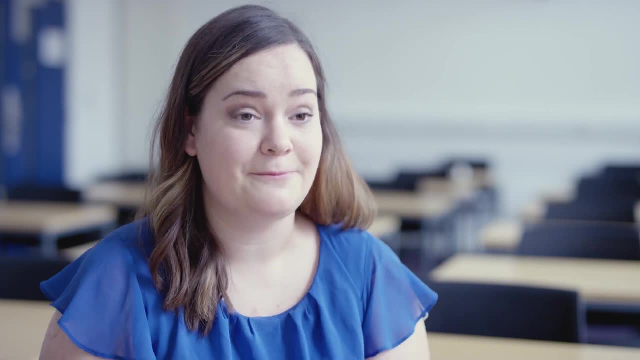 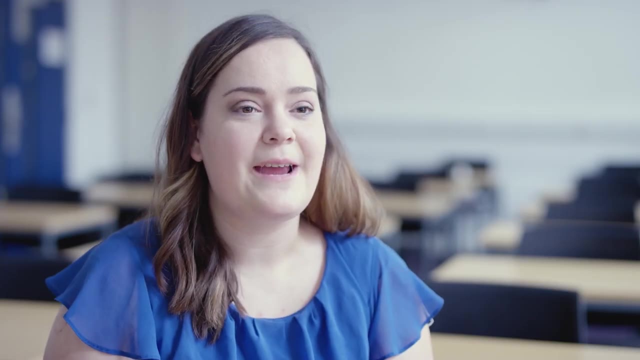 came to us with that problem And we were able to do a lot of research on that, So we're able to solve that problem- and asked us if we could help solve it And we did And because of that, now engines are flying safer, which is not just cool but really inspirational to know that you're making 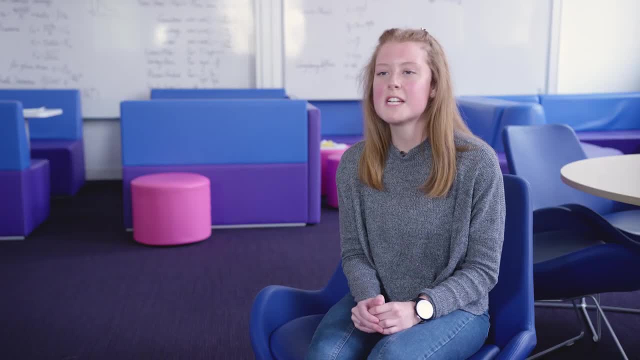 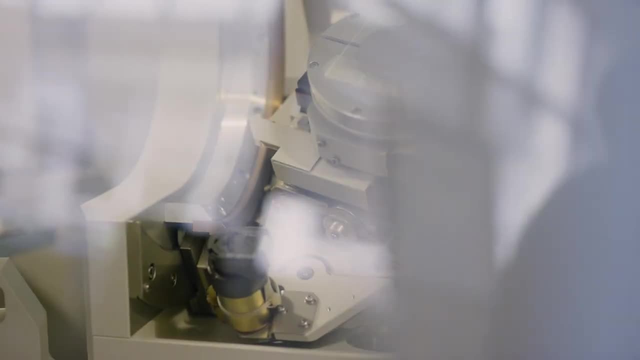 a difference. I really enjoy the course. I love how interactive it is. We have labs every week. It also gets you used to equipment that you could be using for your third and fourth year projects. It's also really nice because everyone's really friendly. You know a lot of people I have got. 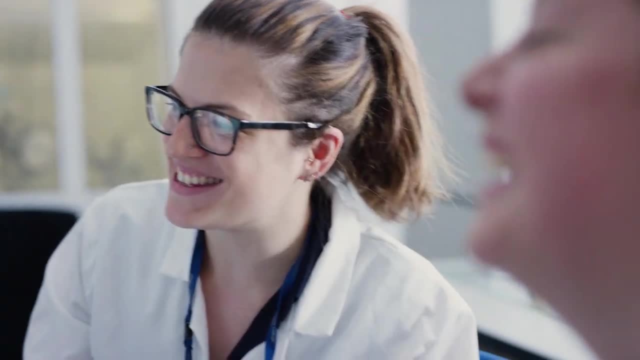 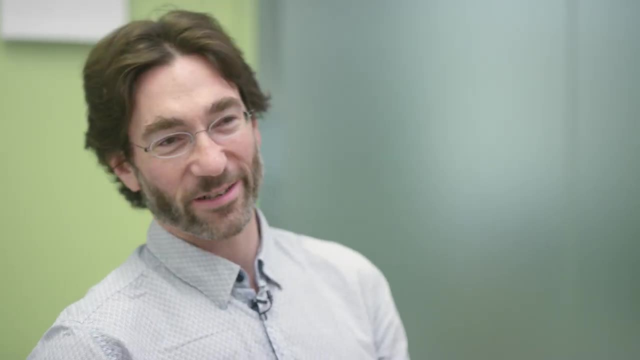 friends in second and third year. If I need any help with work or anything, I can always go to them. There's a great background for very many different kinds of career. Of course, many of our graduates love material science so much. they want to carry on, They want to do research, They want to take. 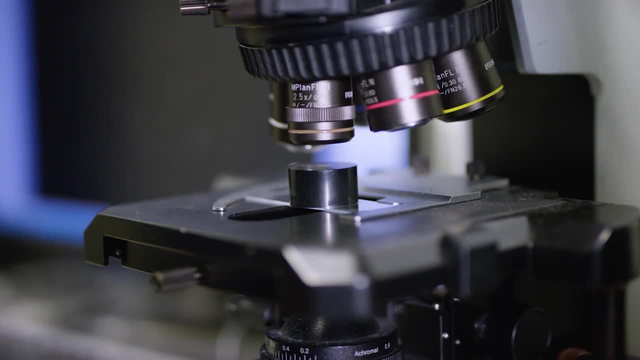 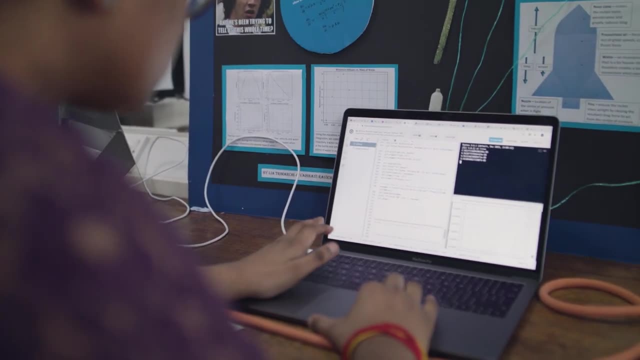 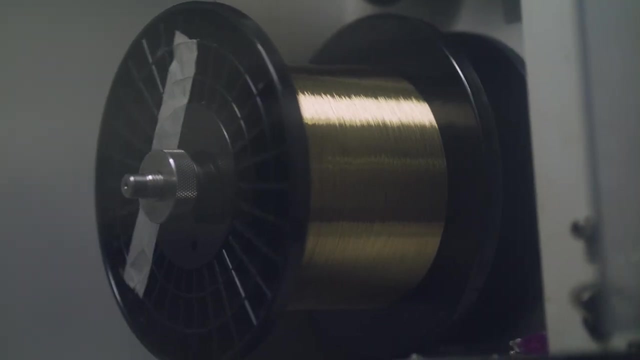 their material science knowledge forward. Other students, of course, take the knowledge they've gained into other fields. Many people go and work in the city, or they work in design or in different engineering kinds of applications. With my materials degree I have plans to become an entrepreneur. I